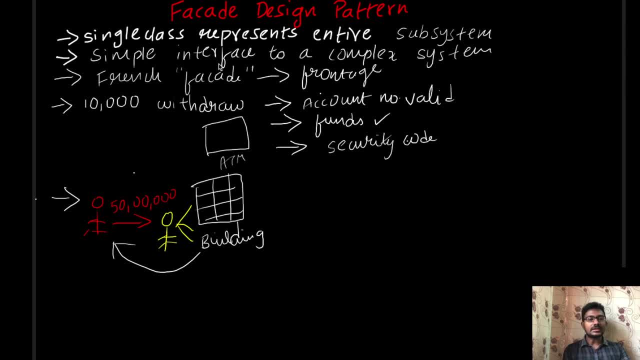 mode to begin the facade in the design pattern is simple interface. simple interface to a complex system. so the system can be complex, but you need a simple interface to operate the operations. so another principle is single class represents entire subsystem. so your system can be, your system can contain n number of subsystems, but the end user should see as a single thing. 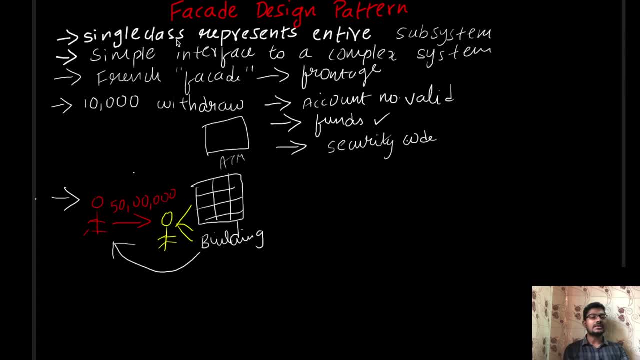 so the entire complexity should be handled by the inner implementation. you don't need to worry about that. so this is the main motto behind the facade design pattern. we can explain that using some real life examples. the first real life example is, if suppose, if you are using atm, if you are trying to withdraw some amount from atm- for example, ten thousand rupees. 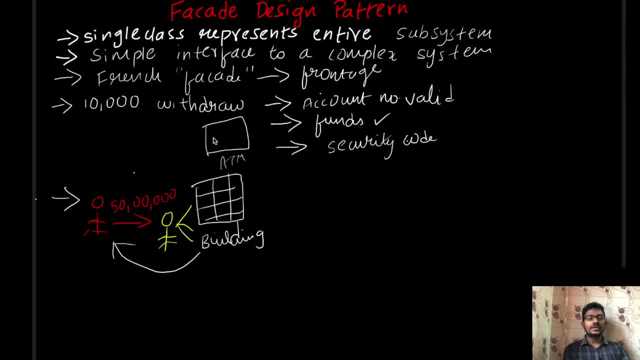 so what you do is you would, uh, you would insert your atm, you would insert your bank debit card into the atm and you would give the required pass, required uh password, which means passcode. so here, once you do that, you know, once you trigger ten thousand rupees withdrawal button, then these are the following things that would happen behind this: 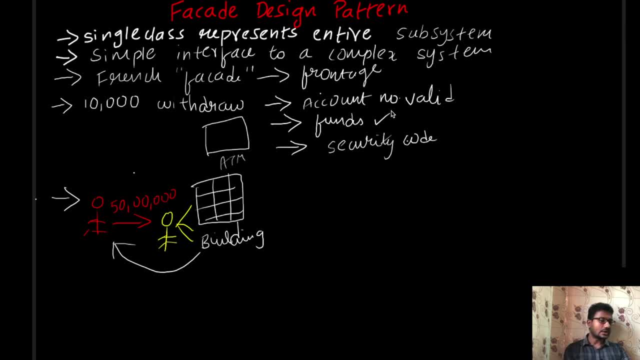 scheme. so first it will check whether the account is valid or not, and then it will check whether you, your account, has some of sufficient funds for withdrawing 10 000 rupees, and then it will check whether your account, your pin code, is correct or not. so after validating all these things, then 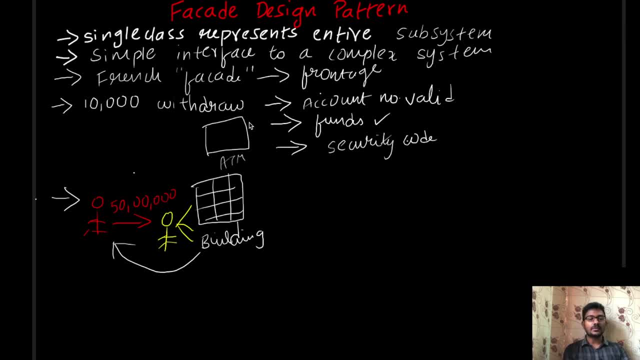 10 000 rupees would be withdrawn from atm. so these are the complex things that handle behind is for the user, for the end user. this interface is very simple. you can just click on some button and you can just give the amount of amount that you need to withdraw. the interface very simple. 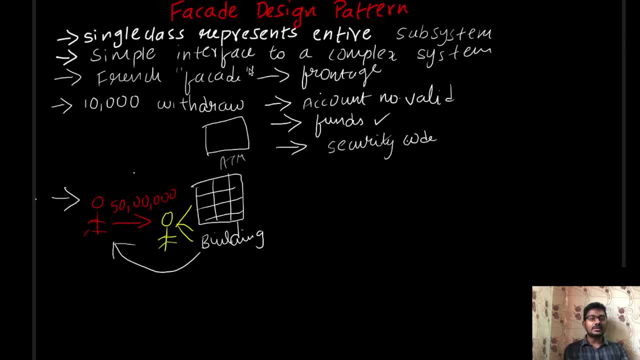 so this falls in the facade design pattern. so simple interface to a complex system. so another example: suppose if you are trying to build a building, so for example, that building consists of 10 floors and each floor should contain some two or three rooms, like that, and then 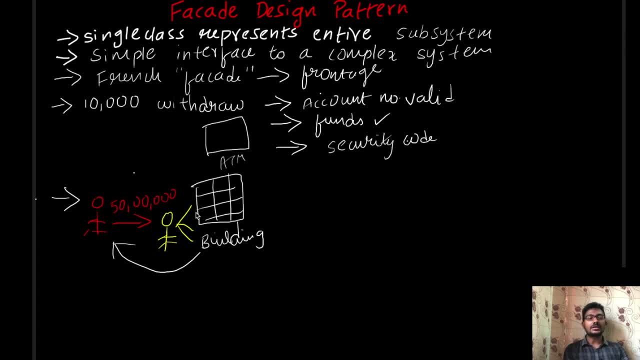 for the quality purpose, you would need to select the better bricks, cement and etc. here you would to build this building. you need to maintain many things and that's a very complex process. so what you are trying to do is you are trying to give this contact to the building contractor. so